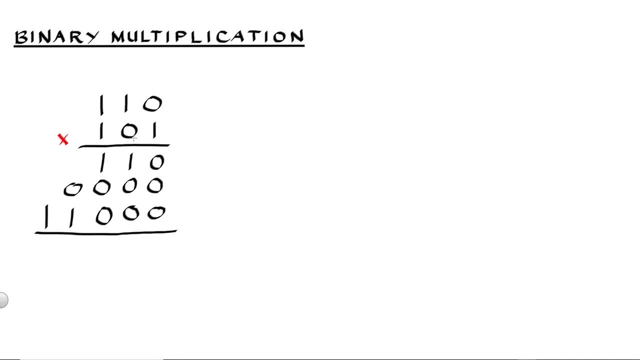 multiplicand. If your multiplier is 0,, obviously you will get 0. Because any number multiplied by 0 is equal to 0. And if your multiplier is 1, you get exactly the same thing: 1,, 1,, 0. Like this one. 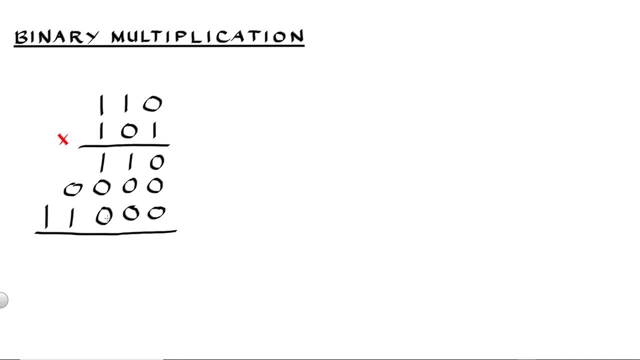 you have 1, 1, 0 and another 1, 1, 0. Then let's proceed to addition: 0 added to 0 is equal to 0, plus another 0 is equal to 0. So we have 1, 1, 0 and another 1, 1, 0. So we have 1, 1, 0 and another 1,. 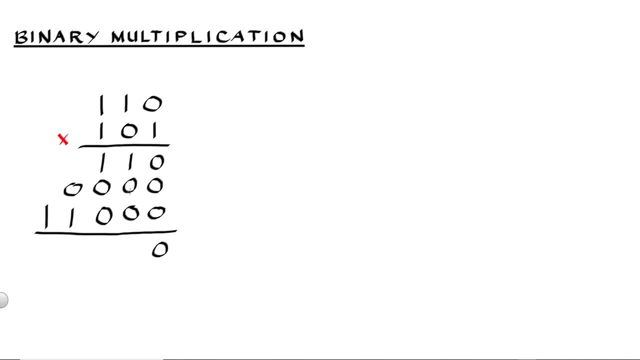 0 is equal to 0.. 1 added to 0 is equal to 1, plus another 0 is equal to 1.. 1 added to 0 is equal to 1, plus another 0 is equal to 1.. 0 added to 1 is equal to 1.. And bring down 1.. So our product is. 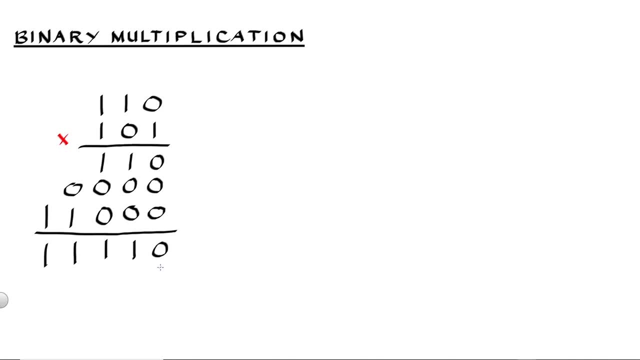 11110.. We can verify our answer by converting the given and the product to decimal. This column is for the ones And this is for the twos. Next is for 4,, 8 and 16.. Then add numbers with the ones. 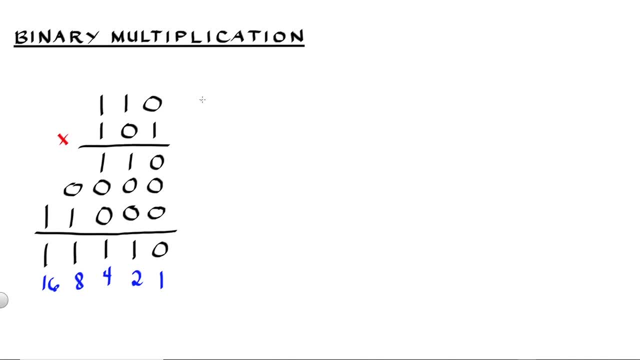 For the multiplicand we have: 4 plus 2 is equal to 6.. And for the multiplier we have: 4 plus 1 is equal to 5. And 6 multiplied by 5 is equal to 30. Then our binary product should be 30.. We have: 16 plus 8 is equal to 24,. 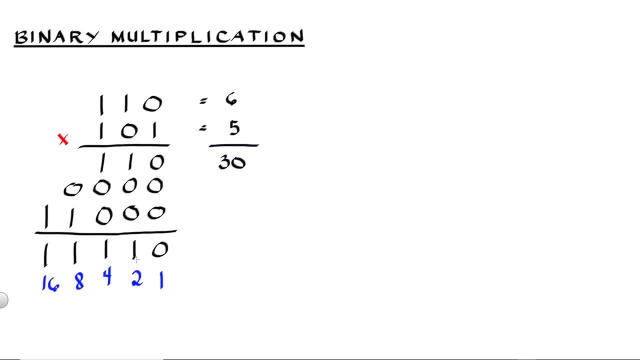 plus 4 is equal to 28 and plus 2 is equal to 30. Then we can say: our answer is correct. For our second example, let's multiply 1, 0, 1, 1 by 1, 0.. 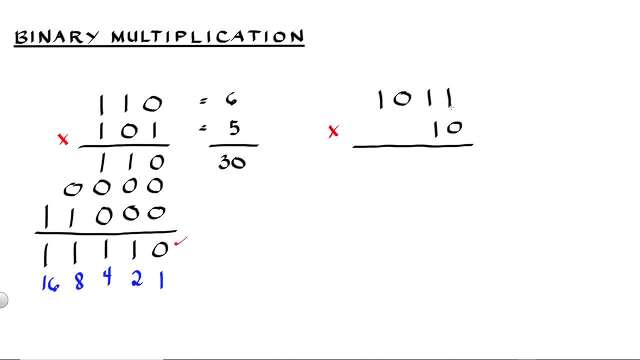 Zero multiplied by 1 is equal to 0.. Zero multiplied by 1 is another 0.. If your multiplier is 0, just fill this row with zeros. So this is zero and this is zero. Next, add another zero: 1 multiplied by 1011.. 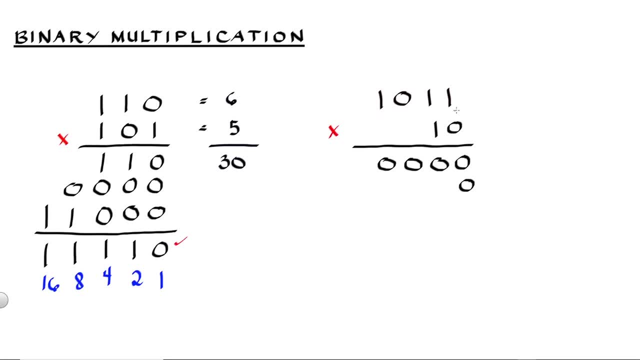 1 multiplied by 1011.. Then we're gonna add another zero, Then we're gonna add another zero. get exactly these four digits so we have one one zero one. then proceed to addition. we have: zero added to zero is equal to zero. zero added to one is equal to one. zero added to one is equal to one. 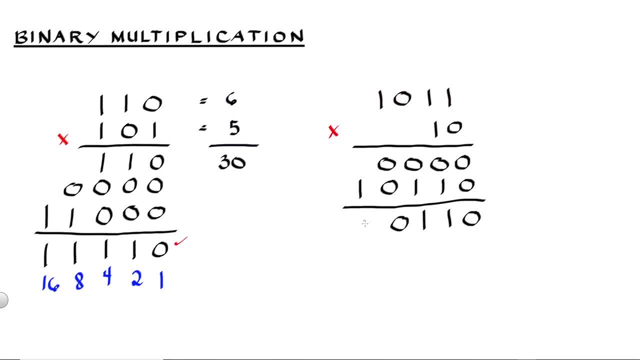 zero. added to zero is equal to zero and bring down one, so our product is one zero, one one zero. to check our answer, we have one, two, four, eight and sixteen. then add up numbers with ones for one zero one one. we have eight plus two plus one is equal to eleven. 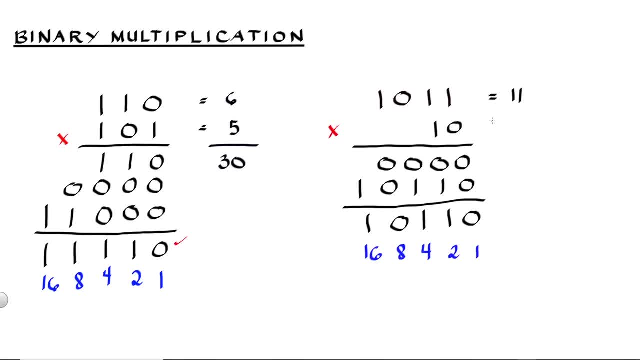 and one zero is equivalent to two, and eleven multiplied by two is equal to twenty two, and our binary product is equal to 16 plus 4 is equal to 20 plus 2 is equal to 22.. so our answer is correct. every time you multiply any binary number by 1, 0 or by 2, all you need to do is add a. 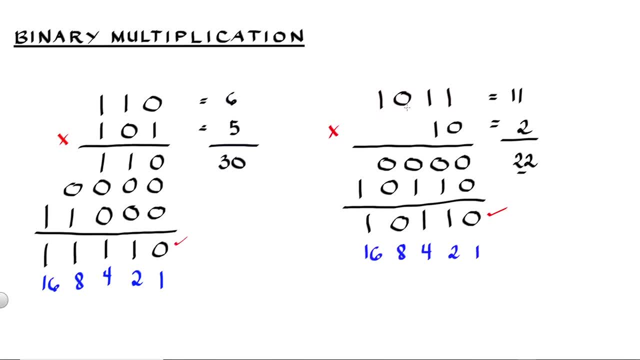 zero. we have multiplicant 1, 0, 1, 1 and multiplied by 1, 0, the product is 1, 0, 1, 1 and 0, so all you have to do is add a 0.. like, for example, 1, 1 multiplied by 1, 0 or 2, the answer is 1, 1, 0, 1 multiplied by 11. 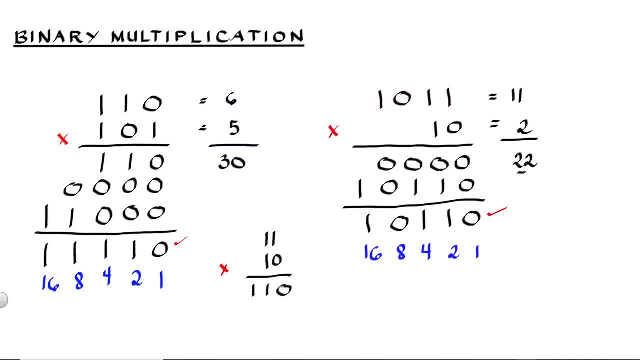 2, 11 and bring down 0, then we have 1, 2 and 4. then add up numbers with 1, so this is 2 plus 1 is equal to 3, and 1, 0 is equivalent to 2, and 3 multiplied by 2 is equal to 6 and for our product, 4 plus 2. 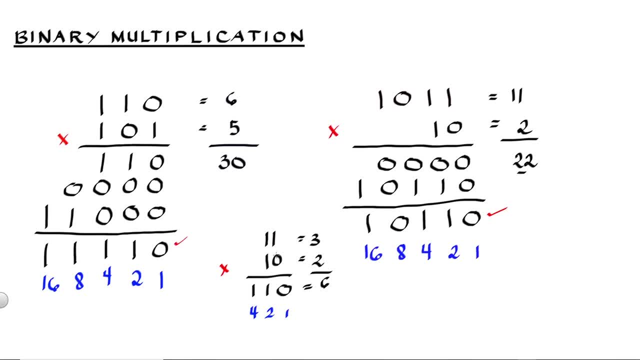 is equal to 6.. so any binary number multiplied by 1, 0 or 2, just add 0.. the same concept as in decimal numbers. every time you multiply a number by 10, all you have to do is add a 0.. like, for example, 15 multiplied by 10. 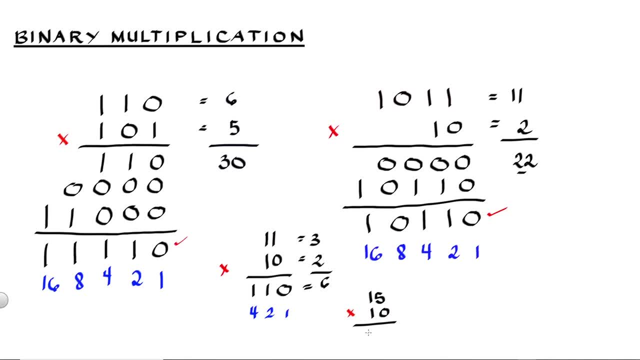 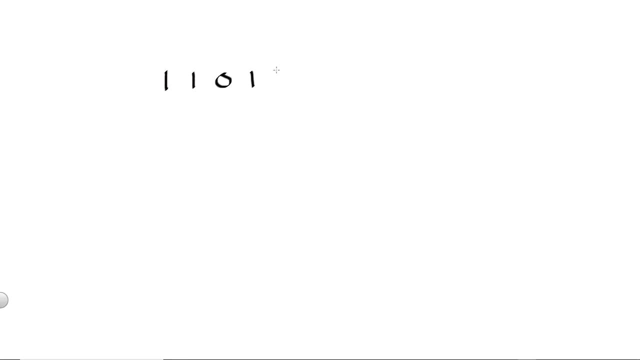 the answer is 1, 50.. all you have to do is add a 0.. 1 multiplied by 15 is equal to 15, and just bring. now let's try a harder example: 1, 1, 0, 1, 1 multiplied by 1, 1, 0, 1. 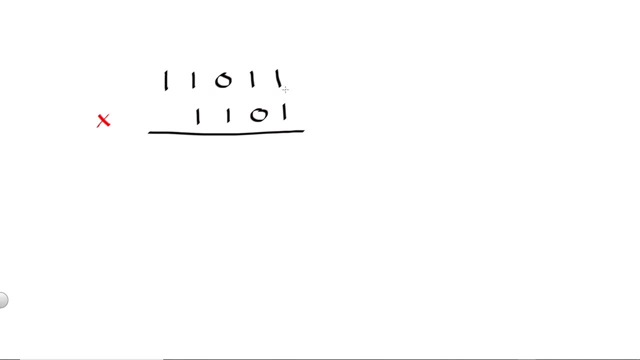 1 multiplied by 1, 1, 0, 1, 1 is going to be whatever is on the multiplicant, so we have 1, 1, 0, 1, 1. then add 0 to go to the next row, and 0 multiplied by 1, 1, 0, 1, 1 is equivalent to five zeros: two, three, four and five. 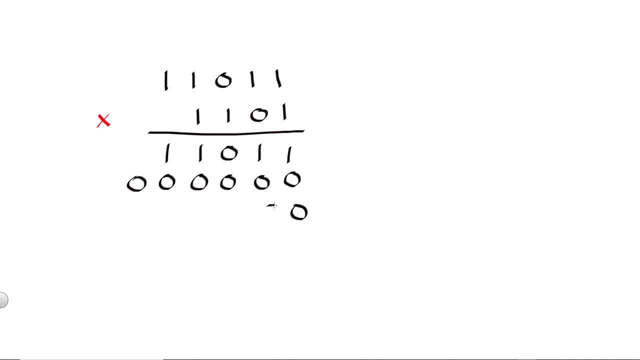 then you need to add two zeros from the right, since our next multiplier is on the third column. then 1 multiplied by 1, 1, 0, 1, 1 is exactly 1, 1, 0, 1, 1. then, to go to the next row, you need to add 3 zeros, since our next multiplier is on the 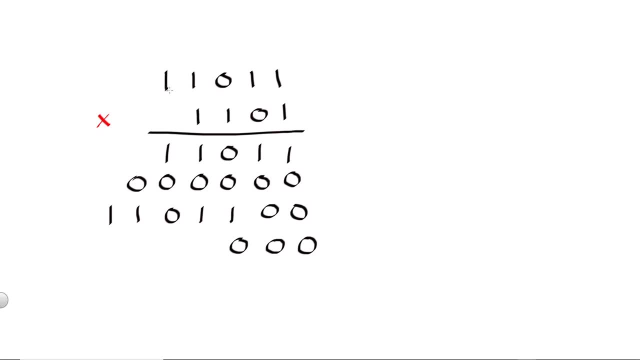 fourth column. then 1 multiplied by 1, 1, 0, 1, 1 is exactly 1, 1, 0, 1, 1. whatever is on the multiplicant, then let's proceed to addition. we have: 1 added to 0 is equal to 1 added to another. 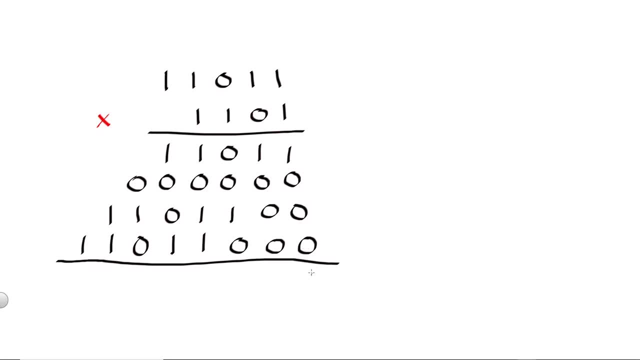 0 is equal to 1 and added to another 0 is equal to 1. 1 added to multiple zeros is still 1, and 0 plus 0 is equal to 0, plus 1 is equal to 1 and plus another 0 is equal to 1. then 1 added to 0 is equal to 1 and added to 1 is equal to 1. 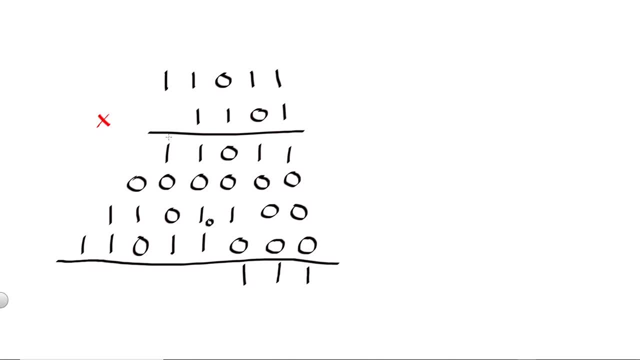 0. so this is 0 and carry 1. then, coming back down, 0 plus 1 is equal to 1. then 1 added to 1 is equal to 1, 0. this is zero and carry one. so zero plus zero is equal to zero plus another zero is equal to zero. 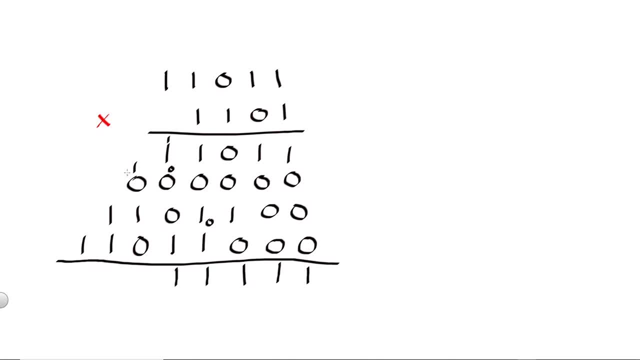 plus one is equal to one, then we have one plus zero is equal to one, then one plus one is equal to one zero. so this is zero and this is one. then zero plus zero is equal to zero. one added to one is equal to one zero, so this is zero and carry one. zero added to one is equal to one, then one added. 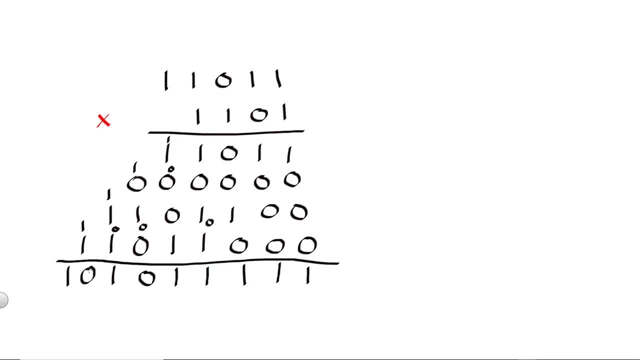 to one is equal to one zero, and let's do a quick check in decimal. so we have one, two, four, eight, sixteen, thirty two, sixty four, one twenty eight and two, five, six. then add up numbers with ones for our multiplicand we have 16 plus 8 plus 2 plus 1. 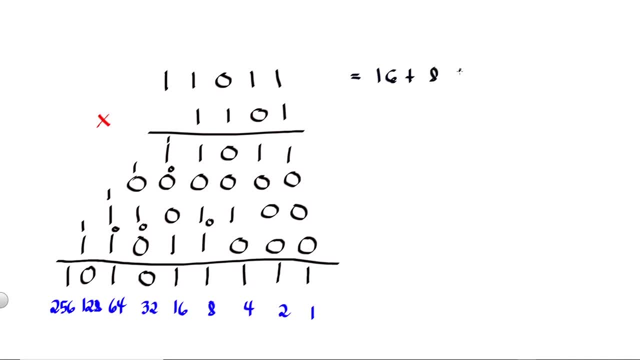 16 plus 8 plus 2 plus 1 is equal to 27, and for our multiplier we have 8 plus 4 plus 1. 8 plus 4 plus 1 is equal to 13. 3 multiplied by 7 is equal to 21. so this is 1 and carry 2.